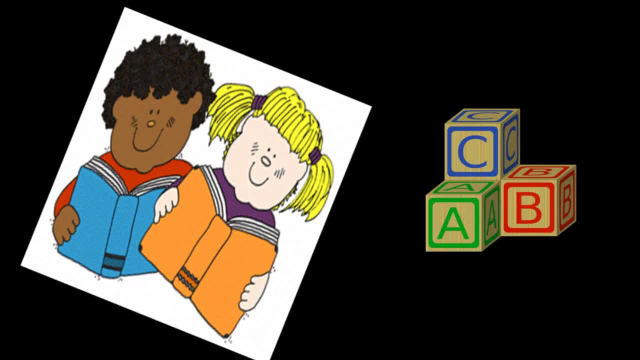 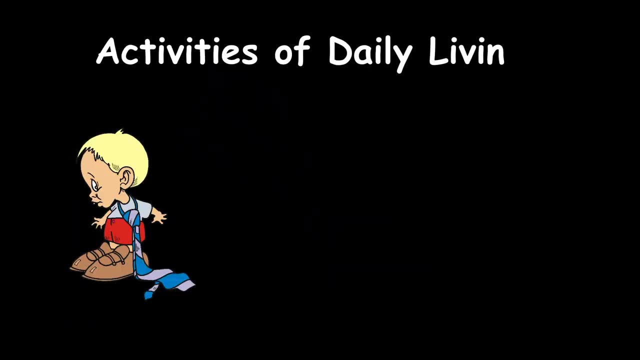 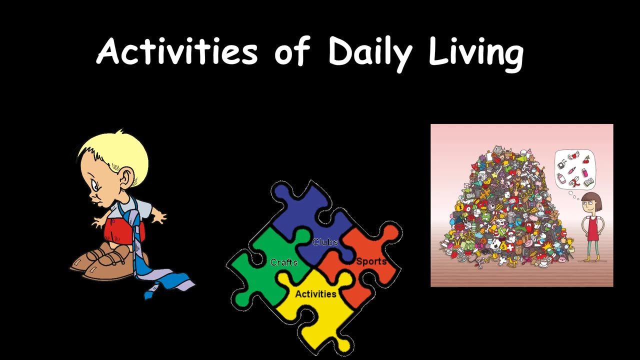 writing maths, we need to make sense of what we are seeing. Cutting, pasting, drawing, coloring puzzles and even while doing our daily activities like dressing, searching for required items for our routine grooming- everything requires visual perception. What if any kid has problem with visual? 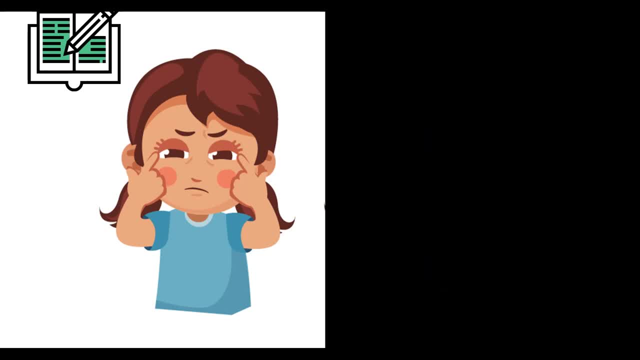 perception and we just let it be, Then their class performance, even the completion of their exams, doing their worksheets, even their handwriting, depends so much on it and will get grossly affected, which of course, will reduce their self-esteem and confidence. So we need to. 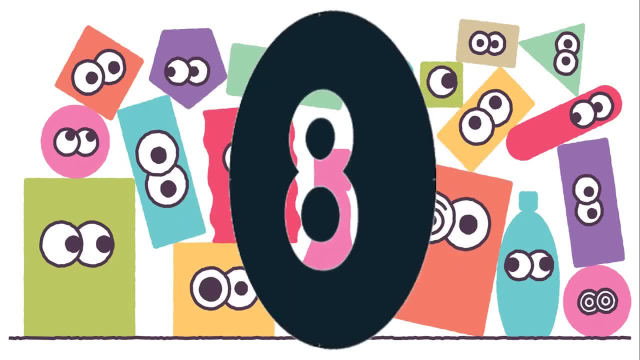 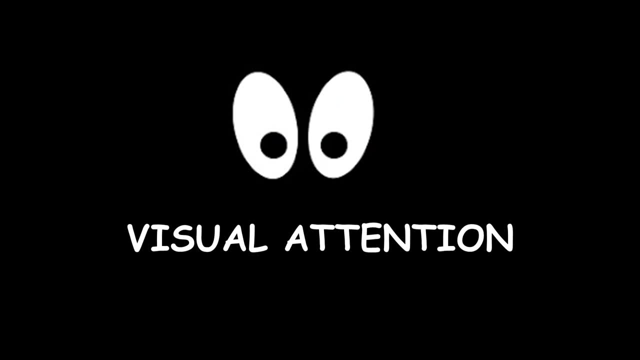 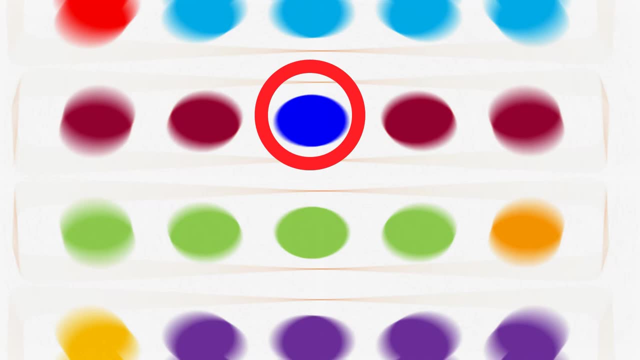 understand how visual perception works. It is done in eight separate parts. The first is known as visual attention, when we simply focus on what is there in our environment and try to filter out the information which seems less relevant. Visual discrimination, when we try to differentiate. 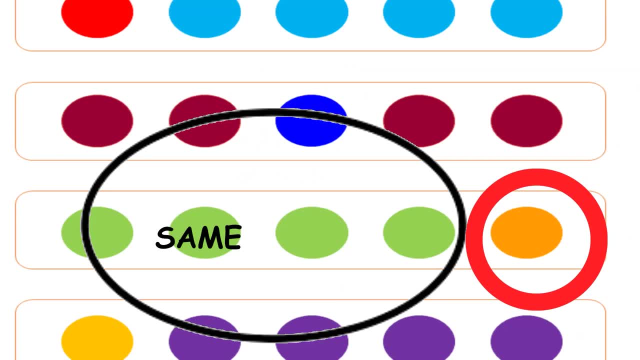 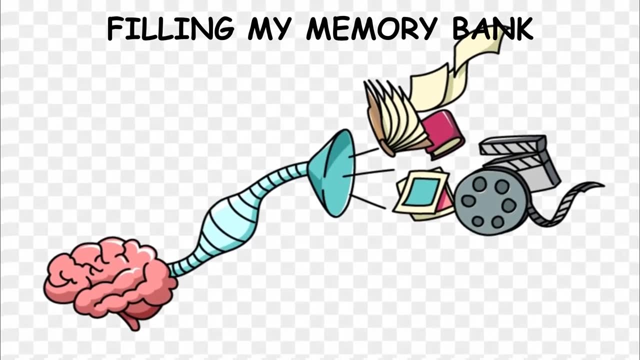 between things or try to filter out the information which seems less relevant. Visual discrimination- when we try to differentiate between things or try to constrain intention to something or try to find similarities between things when it comes to a faceshift- is called visual announcing or identifying anything. 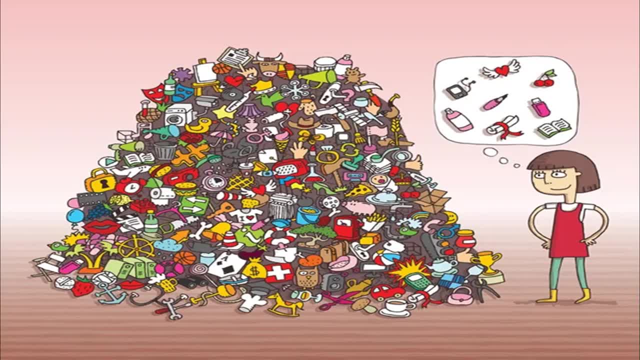 That means when things are necessary or urgent or during something we just stay in order and we endlessly try to see what is in the room. But that does not hallway some sort of potential date. We address the confidence we have to the experience of helping the young and the 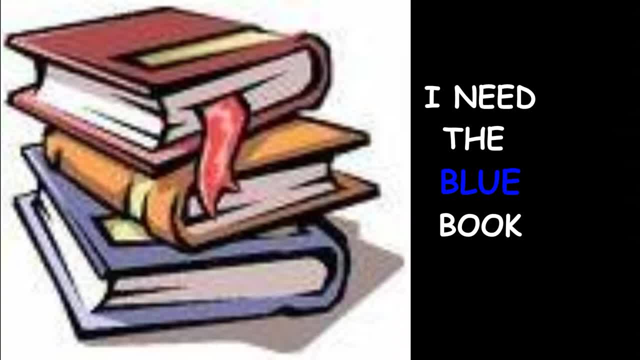 young to face a situation, whether it's there or not, And this is a fighter or not. certainly Visual memory to recall everything we had seen and even if they are in a certain sequence or order, it is visual sequence memory to recall whatever we have seen and if they are in a certain sequence or order, esse called us visual sequential memory. 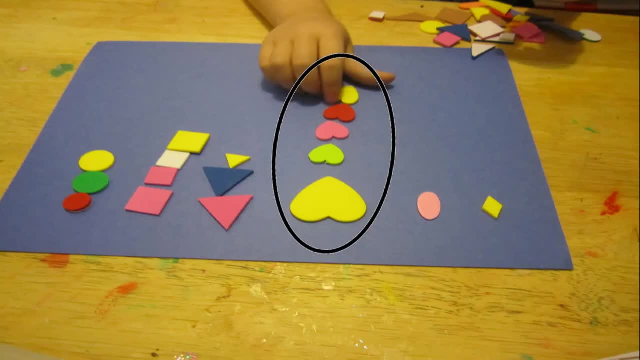 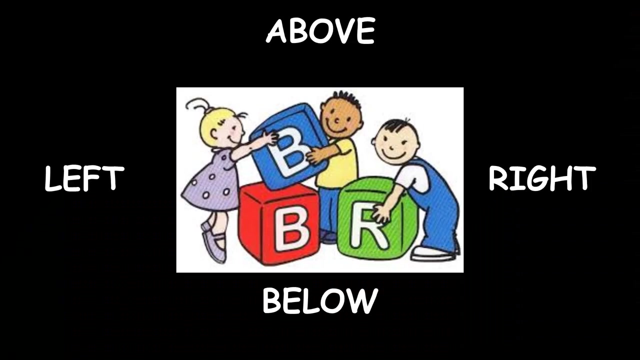 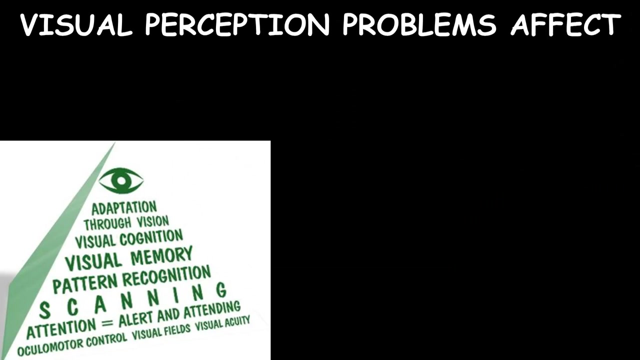 visual closure. we know the forms and shapes of objects, even sometimes when their size or orientation has changed. it becomes visual form constancy. and finally, when we are trying to relate to objects with respect to each other, whether they are above, below, that is, visual spatial relations, the very specific problems that your child can face in visual perception.